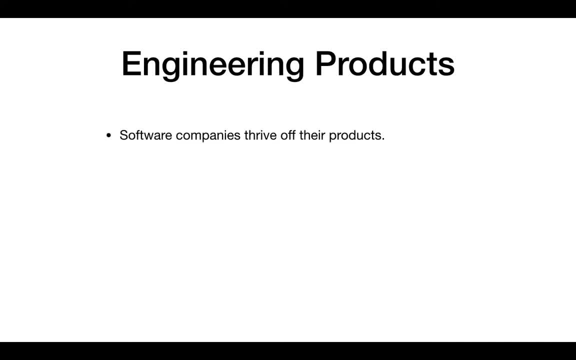 good products. Well, as we all know, software companies thrive off their products. Their product is their lifeblood. If we have a very, very successful project, a very successful product, the software company will attract consumers that like their product and, in turn, 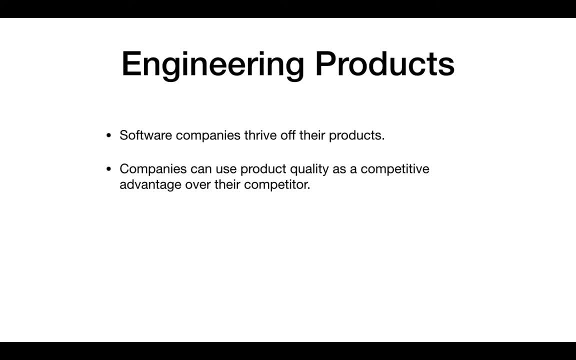 hopefully make money, make revenue, And we can use this as a competitive advantage over the competitor. Now the term product quality or software quality is very vague, because how exactly do we measure quality right? We could have one piece of software that looks: 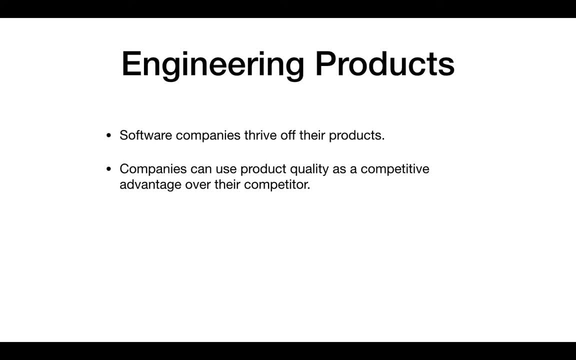 beautiful. It's designed really nicely. The UI is amazing. We have another product. that's a very basic UI and it doesn't look very good, But that basic UI and that basic project could be releasing features day after day, day after day of updates, while the very nice looking product is releasing features. 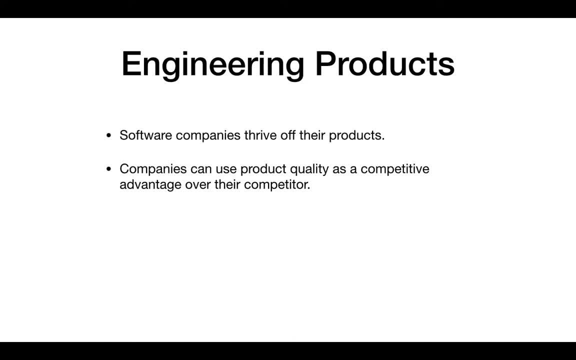 after a month, right, And there could be just simple ones which were done in a day in another product. So that's one metric of quality we can use And that's maybe a marketable advantage over the competitors, And we want this so that we can. 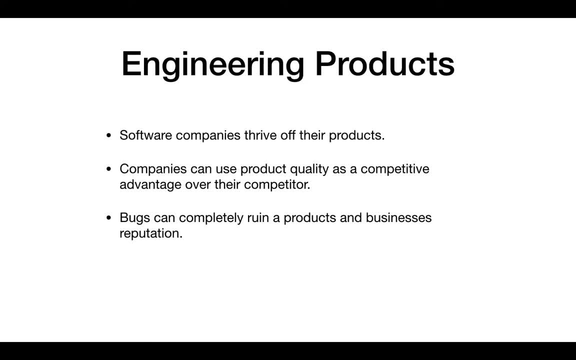 avoid bugs, right? So bugs are a sign of low quality software, Not one bug, a few dozen bugs which really ruin the experience of a product And this could damage a business's reputation. So obviously we want to avoid this. So we want high quality software and 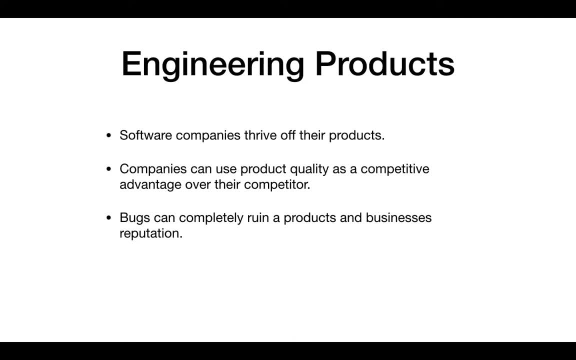 we want to minimize bugs as much as possible And really to achieve high quality software, we need to achieve high quality building the software. So we need a high quality software. So we need to achieve high quality building the software. So we need to achieve high quality. 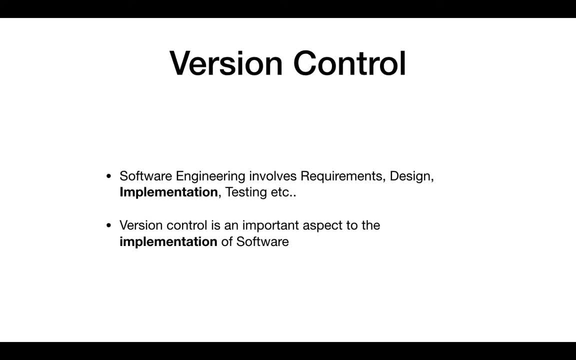 building the software. So we need to achieve high quality, convenient software. But really, you know, we had to do it and then we have to the, which is basically our software engineering process. So the software engineering process is defined in many ways. The definition I'm going to go with here is: you know, we've got the requirements. 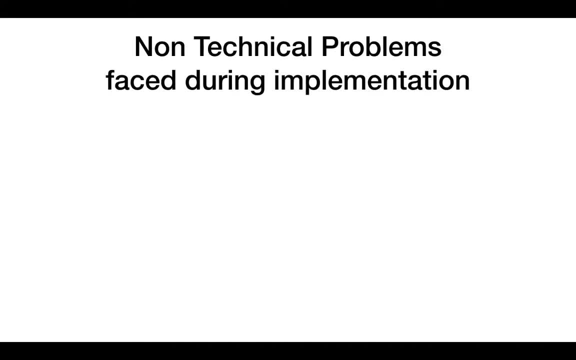 phase. we've got the design phase, invitation testing, etc. And version control falls under the implementation aspect of software. So, along with writing our code, we're going to be using technical problems. well, I want to be able to experiment with features without ruining. 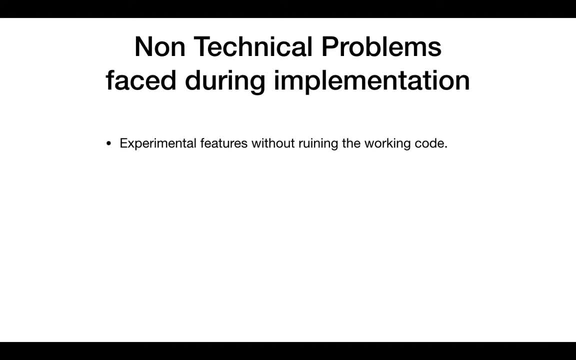 the working code. So write some code without breaking the working code that exists. I want to be able to also trace the origins of bugs that I didn't encounter from before. In doing so, I can find out when it happened and where it happened and in what context. Collaboration. 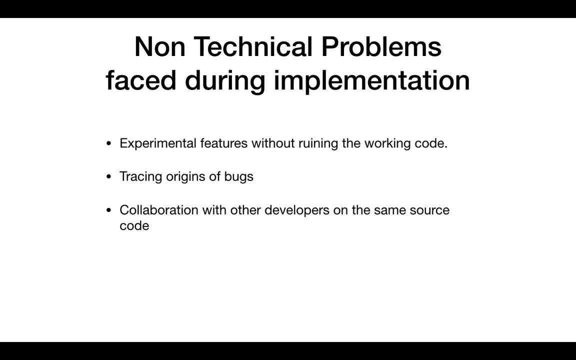 with developers as well. that's a very common problem in software projects. So how can I collaborate productively with other developers on the same source code so that we can split up the work and they can do this and I can work on this particular problem? And finally, 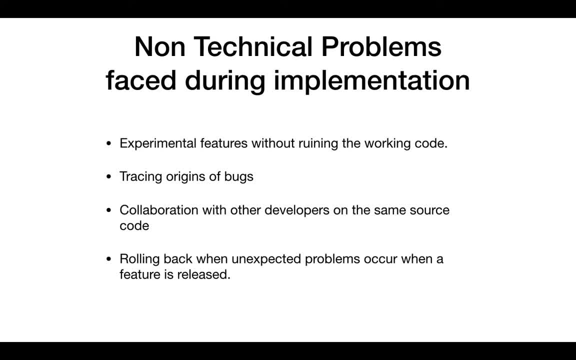 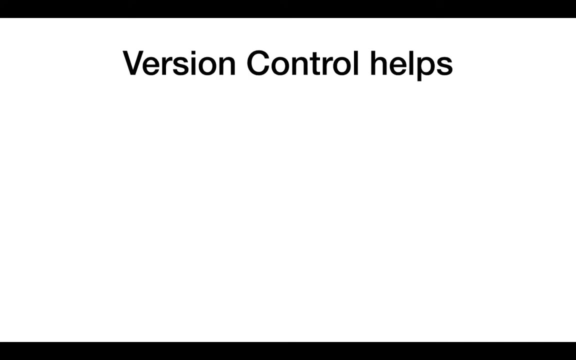 I want to be able to. how can I roll back to a previous version or to a previous working version of my software or my product when an unexpected bug occurs? This could happen in the future. So rolling back is a problem we face during implementation. So version control helps. 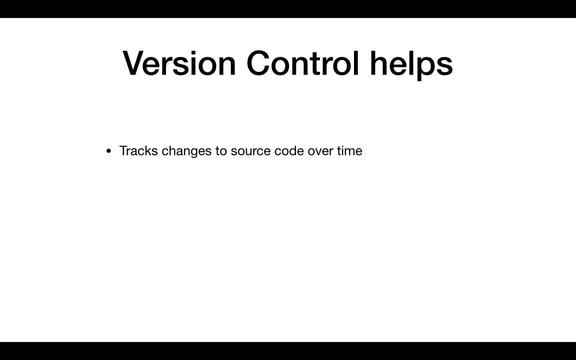 in all those aspects We can track changes to our source code over time. That's kind of the fundamental existence for version control. So because we can track changes to source code over time, we're able to roll back to previous versions of code. We can view a complete 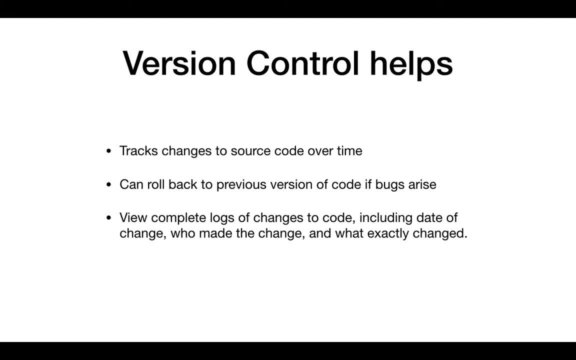 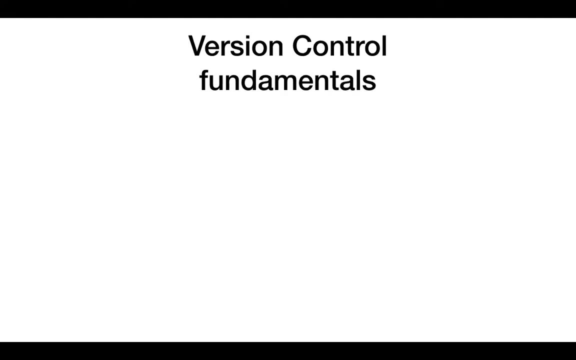 log of changes to the code, including the date of when changes were made, who made the change and what exactly was changed. And version control also enables productive code collaboration, So it goes a long way to providing collaboration. So now let's take a look at the fundamentals. 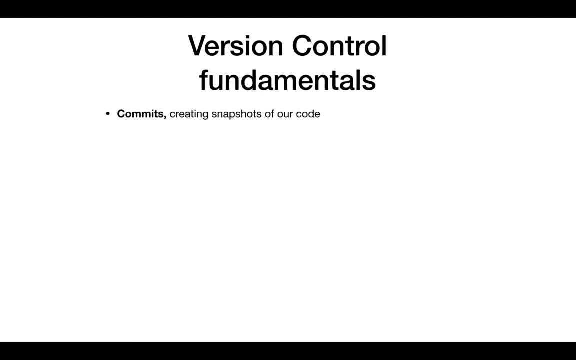 of version control. The most fundamental concept we need to understand is the concept of a commit, which is essentially a snapshot of our code. So if we want to make a change, we need to take a picture of what our code looks like at a current point in time. Now, what code do we mean? Well, that's what we mean by tracking. 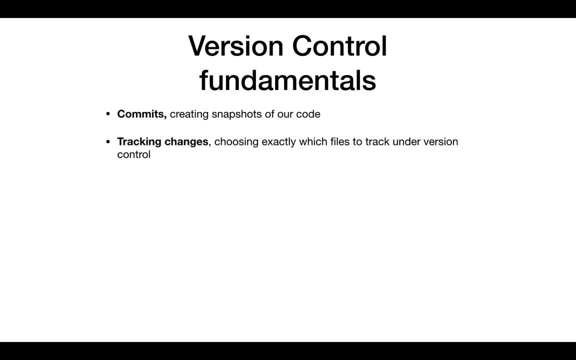 changes, I'm able to choose exactly what files I want to keep track of, or I want version control to keep track of, such that we can create commits and snapshots for that code. And now, as a result, because I'm creating multiple commits for the same bit of code, or for the same files, then I'm able to view change logs and view essentially the same files which I'm able to keep track of. So there are two ways to keep track of files. The first way is to use the version control and the version control to see if there's any. 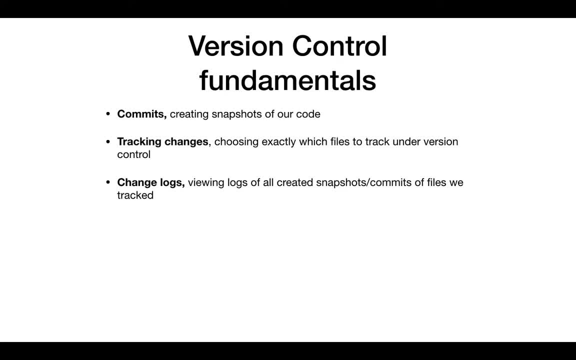 errors, or if there's any errors that you have, or if there's any errors, that you can see logs and view a series of commits of all the changes we made, all the snapshots we made for our code. Also, I want to be able to do what's called merging and branching. 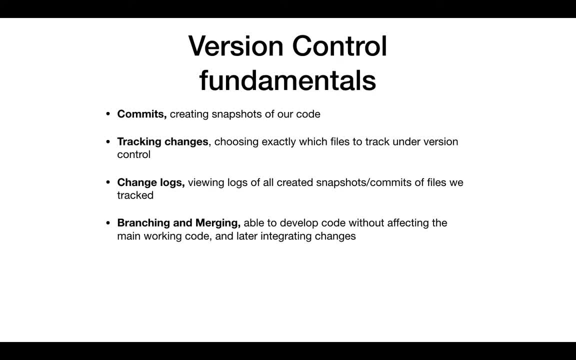 In other words, I want to be able to branch off of my main code and able to work in isolations, allowing me to work on experimental features, And then I want to be able to diff, or I'm diffing, or seeing a differential between 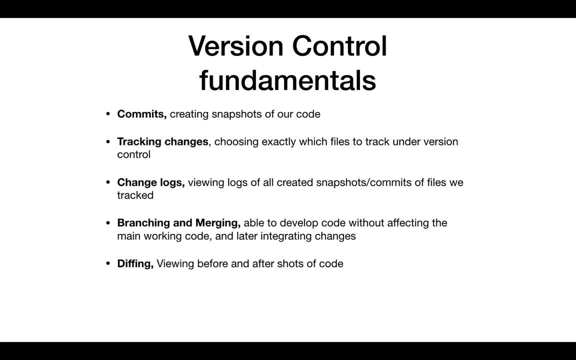 a before and after version of my code. So if I've added 100 lines of code, I want to be able to see a before and after view of that code, so I know what exactly I'm adding. And finally, to enable collaboration, I want to be able to resolve conflicts between multiple 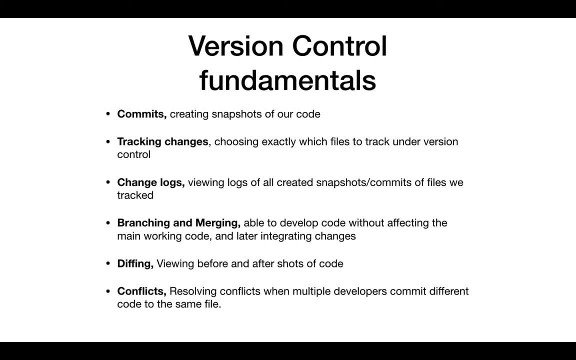 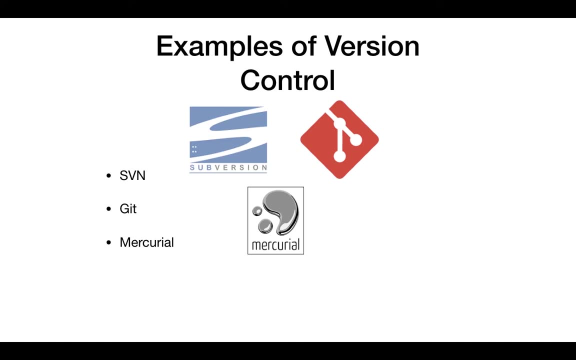 developers who are contributing maybe to the same file and have edited the same function. I want to be able to resolve those conflicts productively so I can keep working on the project. Okay, So those are our fundamentals laid down and all these examples of version control kind. 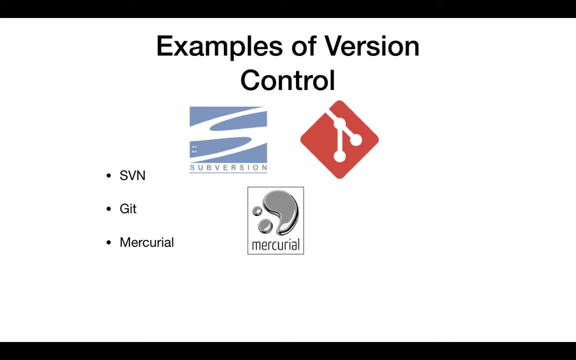 of implement those fundamentals. So we've got subversion, we've got Git and we've got Merkle. All of these kind of implement those fundamental principles that I mentioned earlier in their own unique way and are used by developers in many different ways. 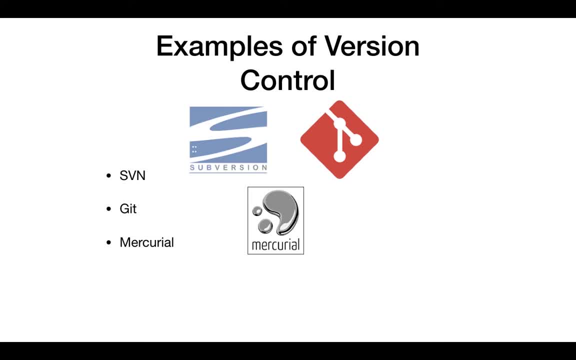 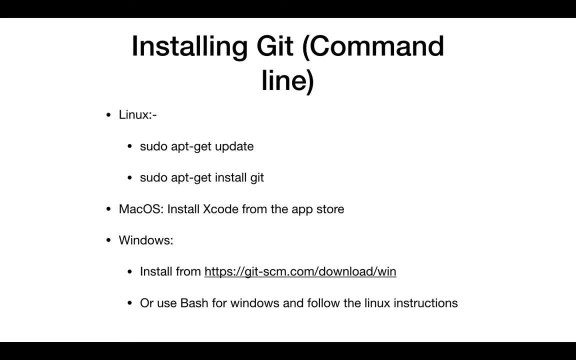 A project will usually use one version control, But it's not completely uncommon to see multiple different version control using, especially if it's an older company who might have used an older version control system such as subversion. Okay, So we're going to be using Git in the course and to install Git, I'm going to walk through. 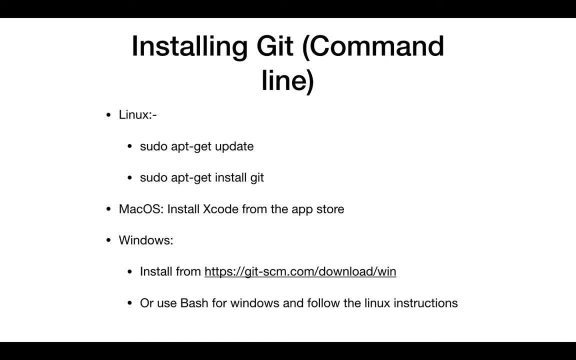 the three main operating systems with installing them. So for Linux, just run those two commands on one after the other. So do a sudo apt-get update, followed by a sudo apt-get install git, And we should have Git installed on Linux. For Mac OS, go to the App Store and install Xcode. 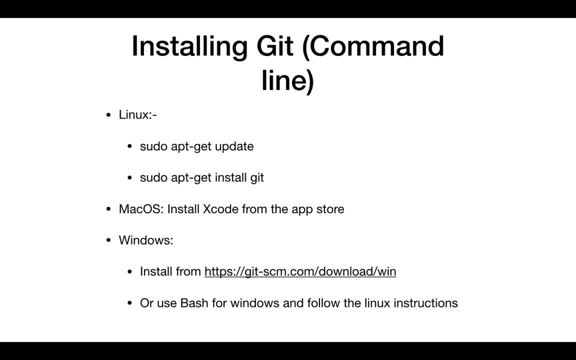 It's around a five to six Git install, so it is quite large. And for Windows, go to the App Store and install Xcode. It's around a five to six Git install, so it is quite large, And for Windows you can go to either this link or you can install Bash for Windows from.